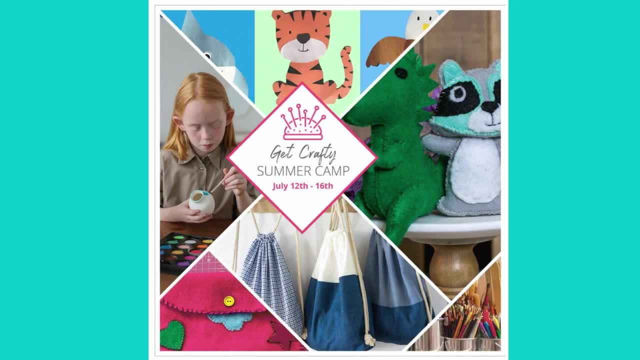 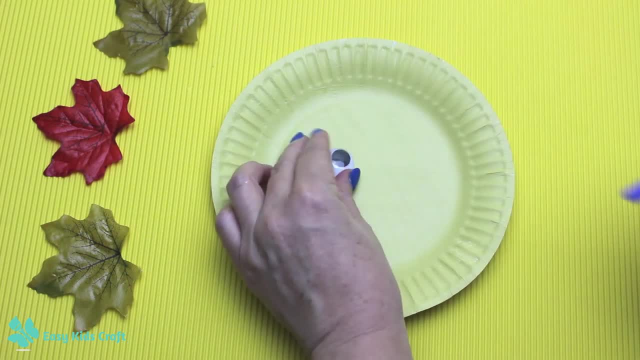 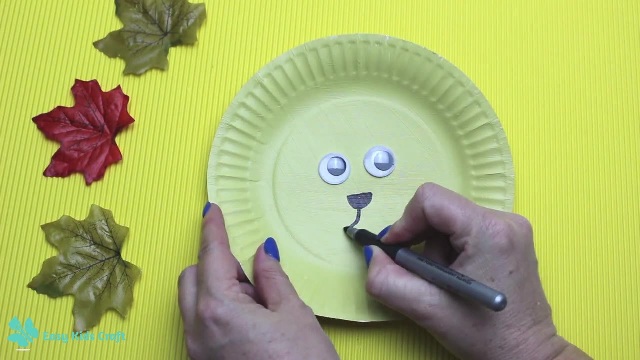 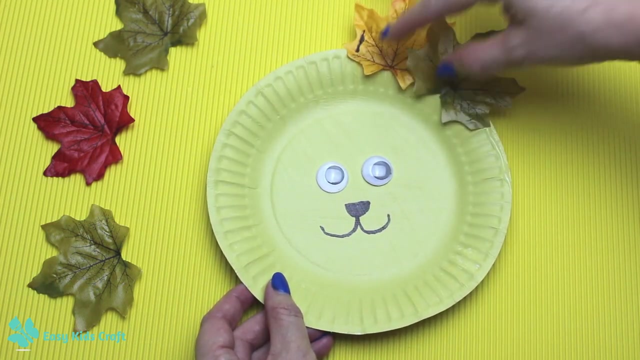 is on the 15th of July. I hope to see you there. Now let's get started. Hello everyone, welcome back to Easy Kids Craft. Today we'll be looking at five easy summer camp craft ideas. But before we start, I just wanted to share a special project I've. 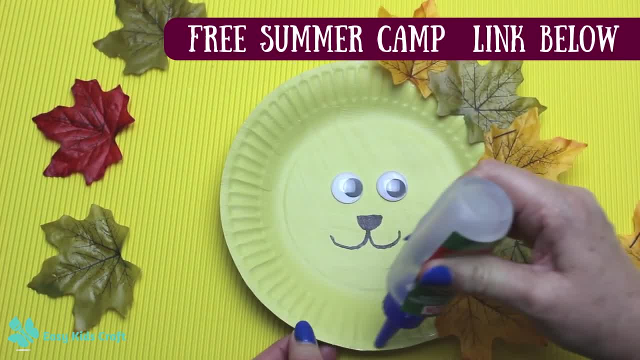 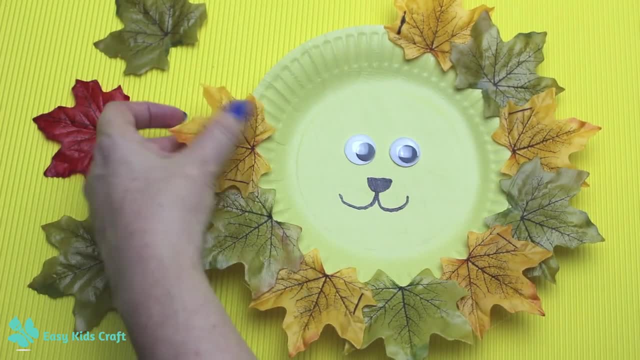 been working with Rebecca Page on the Get Crafty Summer Camp. This free virtual camp includes over 40 craft classes from around the world for children between 5 and 12 years old, including one taught by me. So click the link below to join. Be quick, as my class 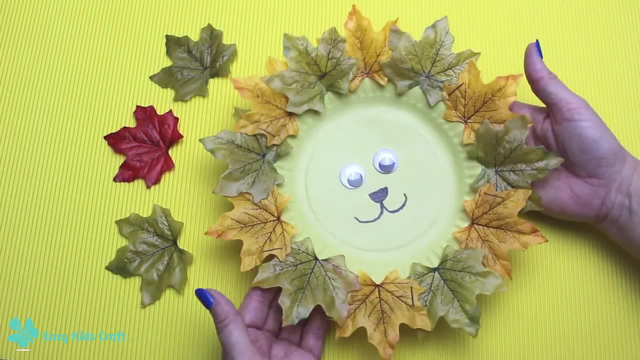 is on the 15th of July. I hope to see you there. Be quick, as my class is on the 15th of July. So click the link below to join. Be quick, as my class is on the 15th of July. 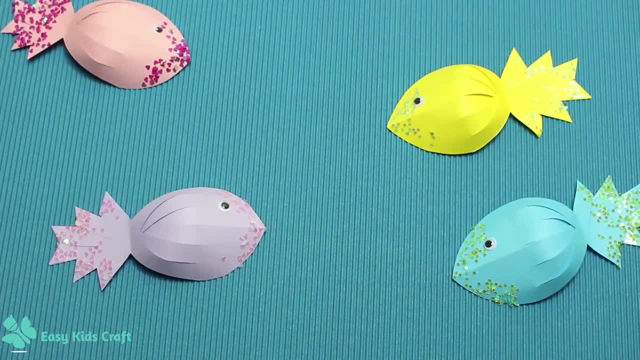 This free virtual camp includes over 40 craft classes from around the world for children between 5 and 12 years old, So click the link below to join. Be quick, as my class is on the 15th of July. This free virtual camp includes over 40 craft classes from around the world for children between 5 and 12 years old. 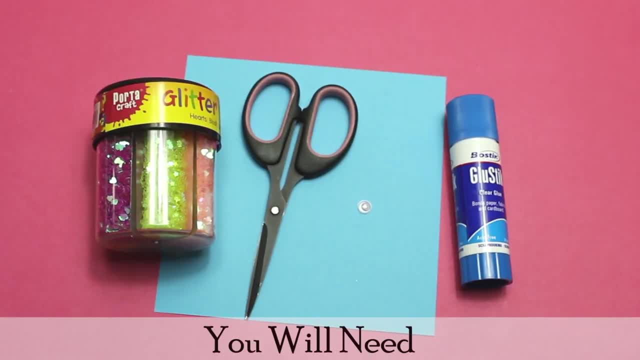 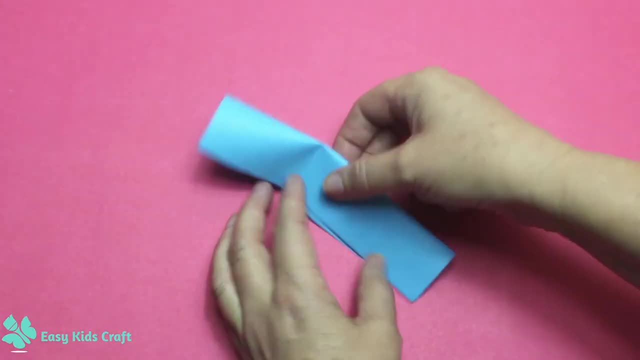 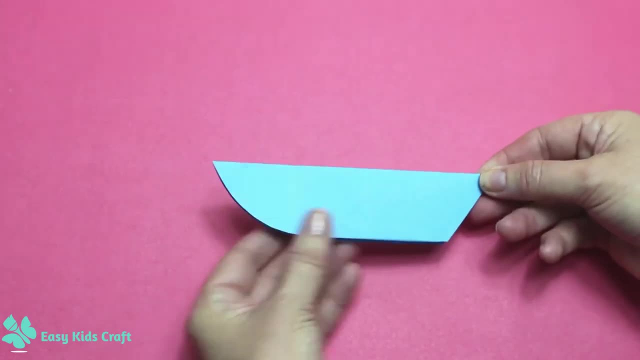 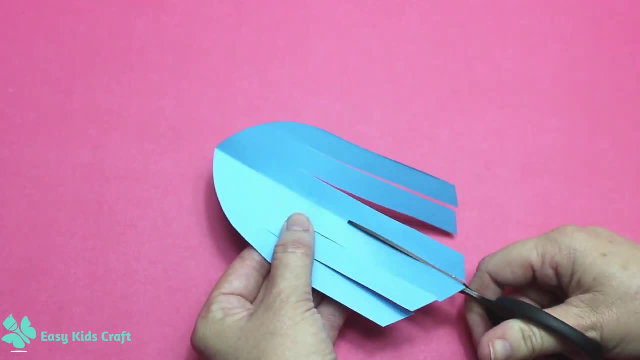 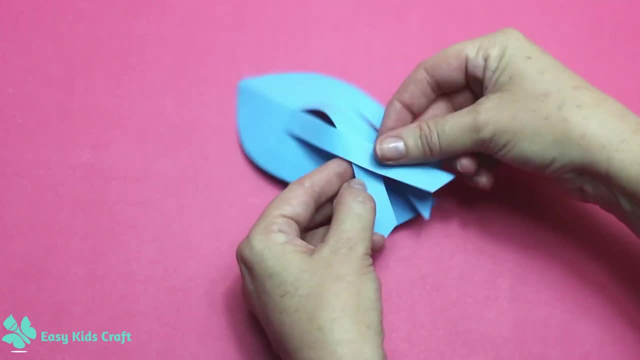 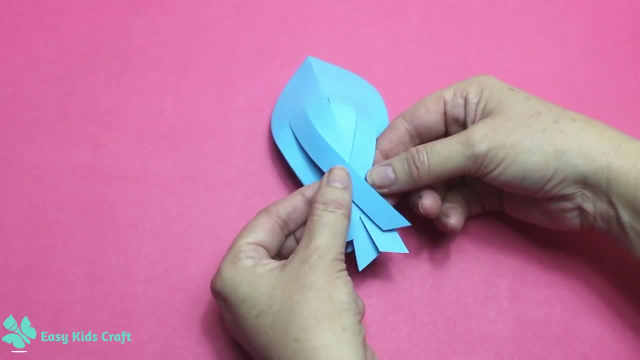 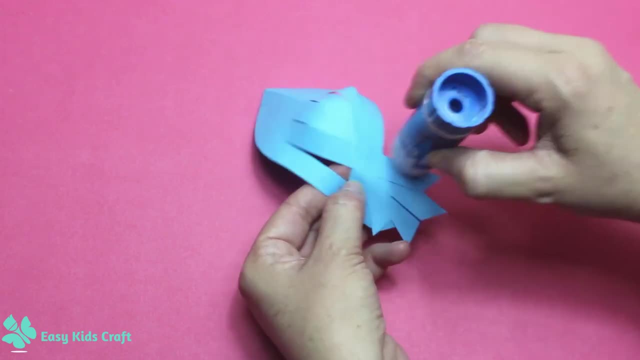 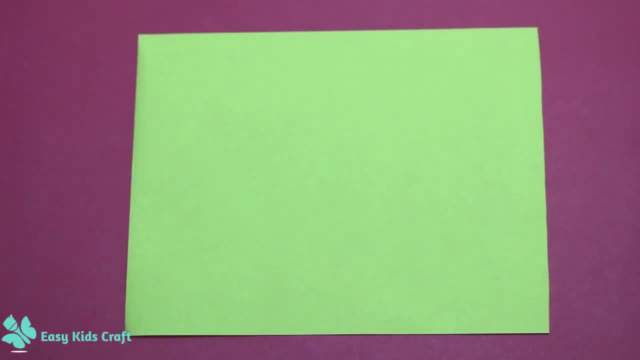 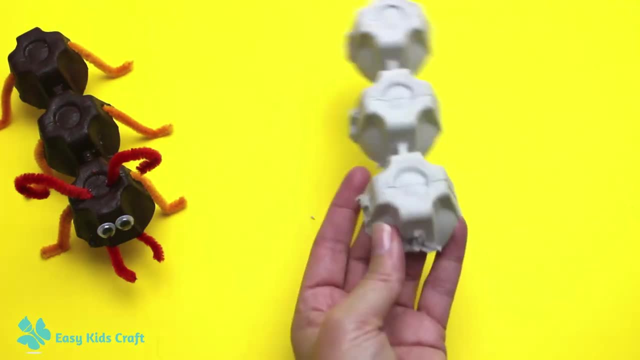 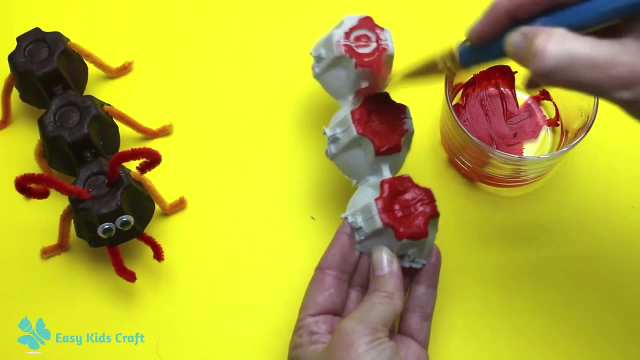 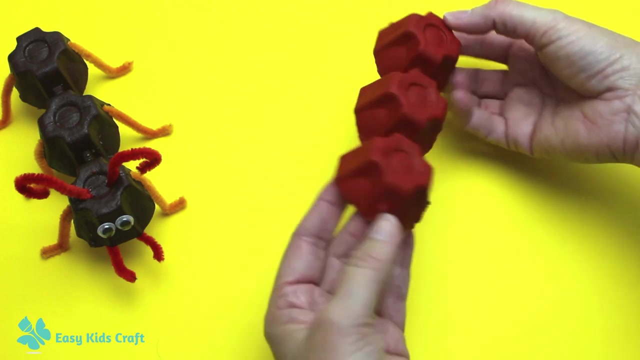 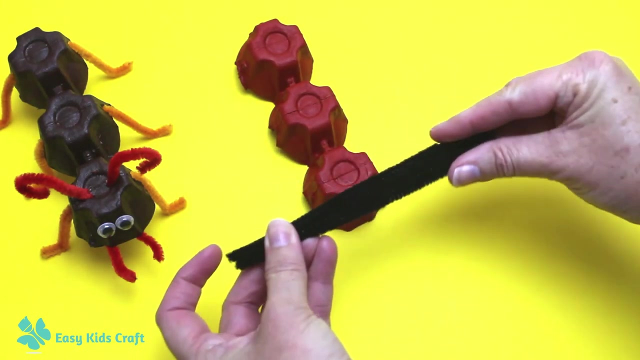 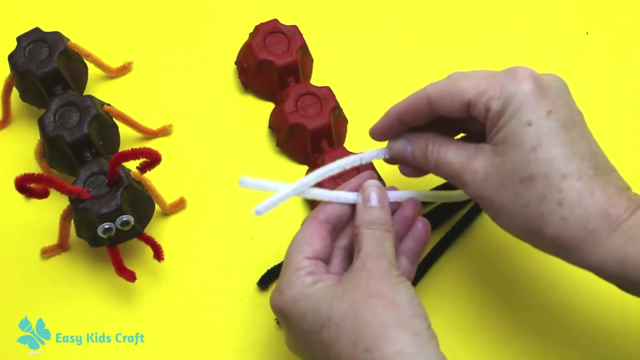 This free virtual camp includes over 40 craft classes from around the world for children between 5 and 12 years old. This free virtual camp includes over 40 craft classes from around the world for children between 5 and 12 years old. Thank you. 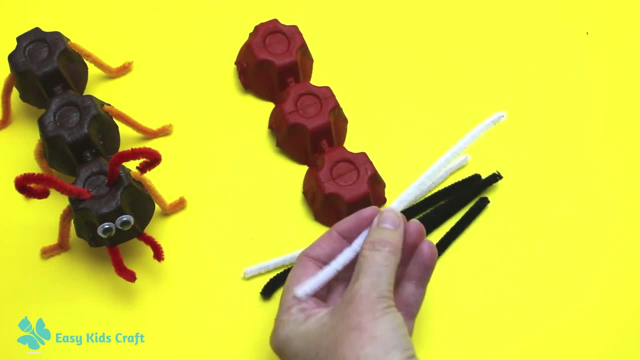 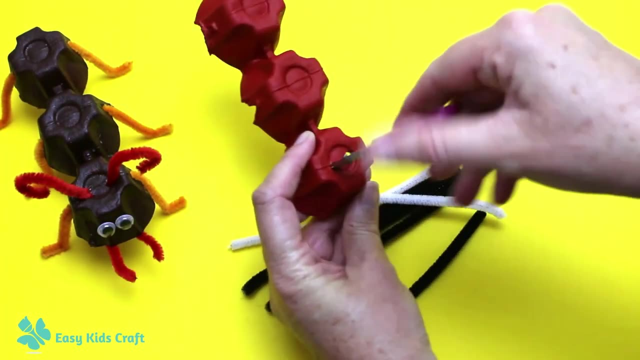 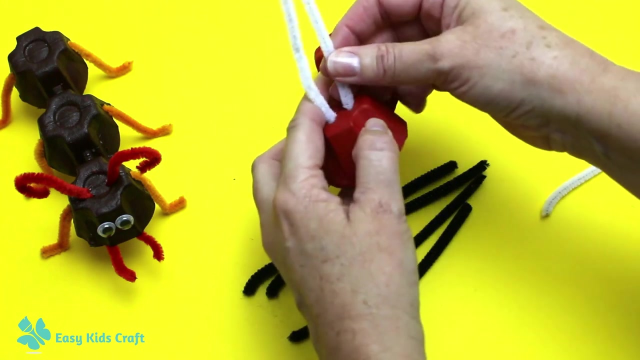 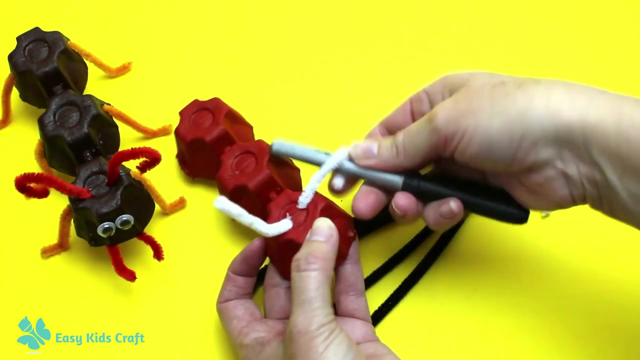 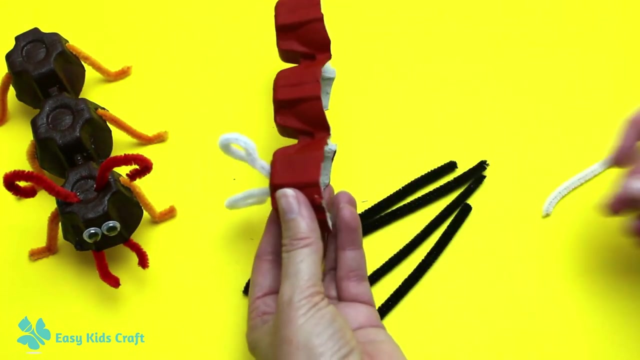 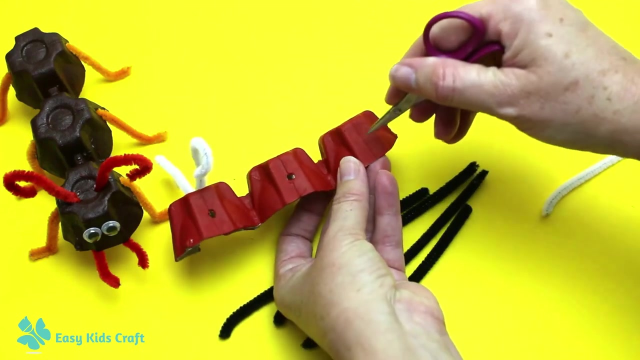 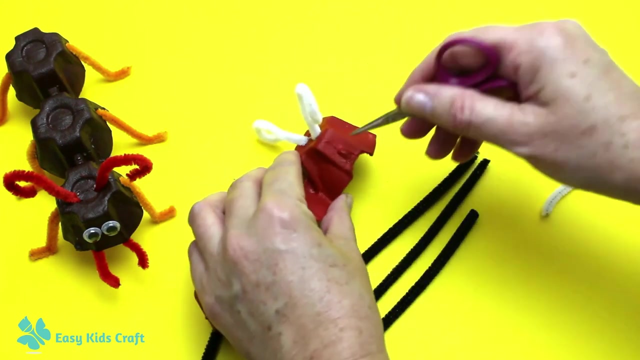 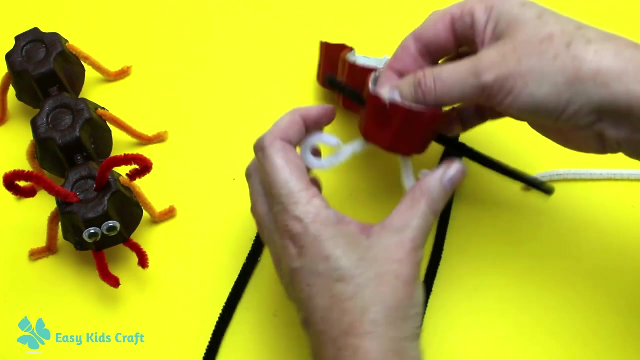 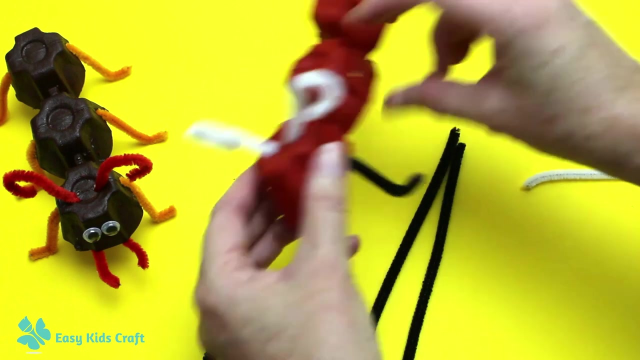 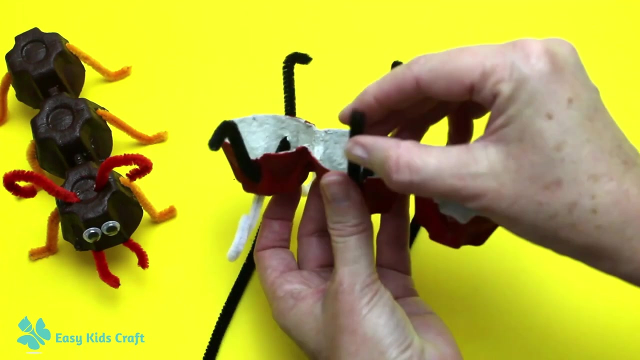 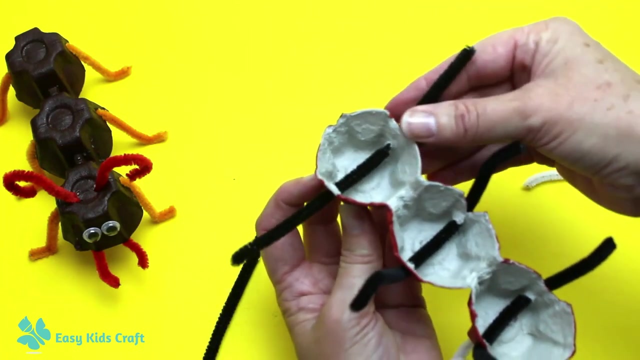 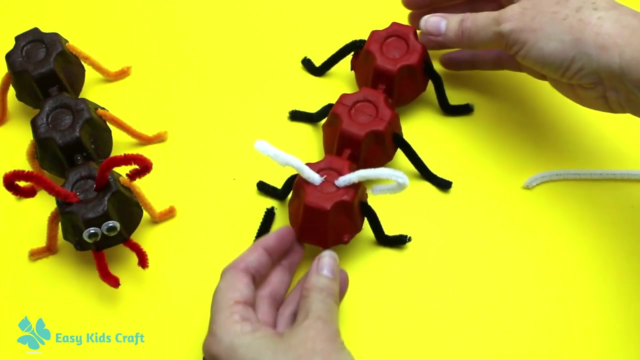 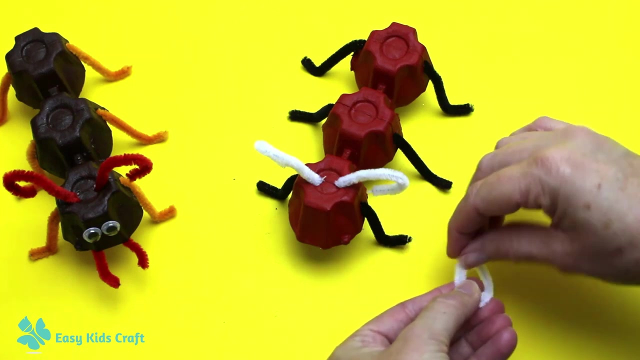 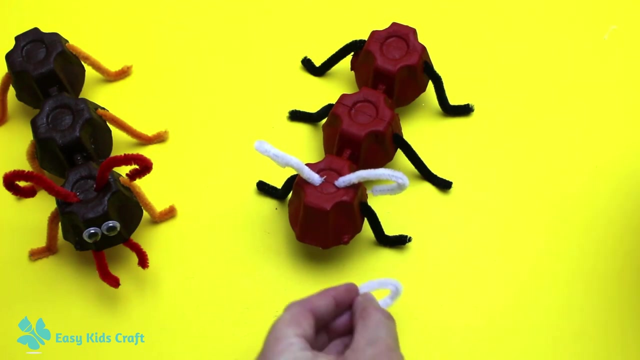 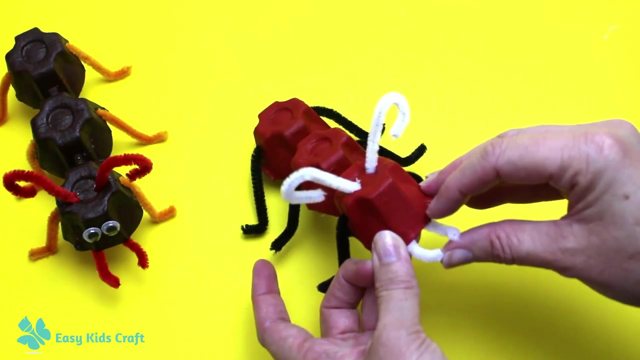 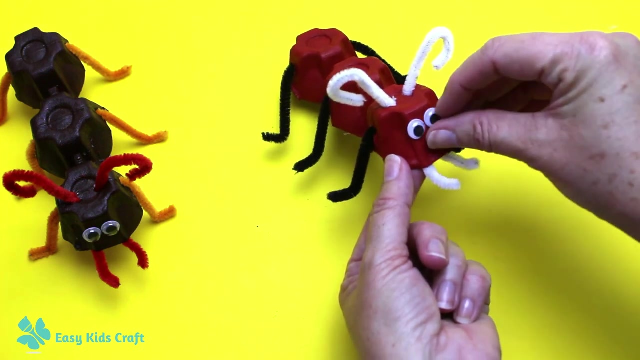 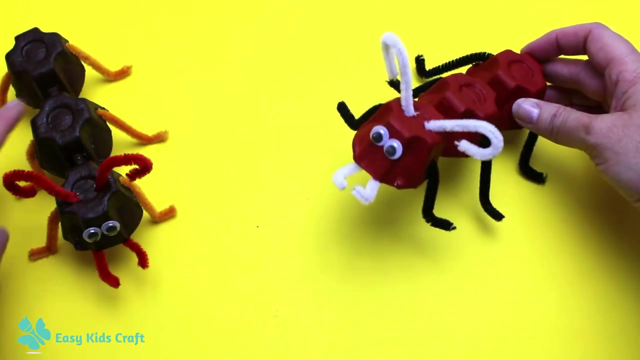 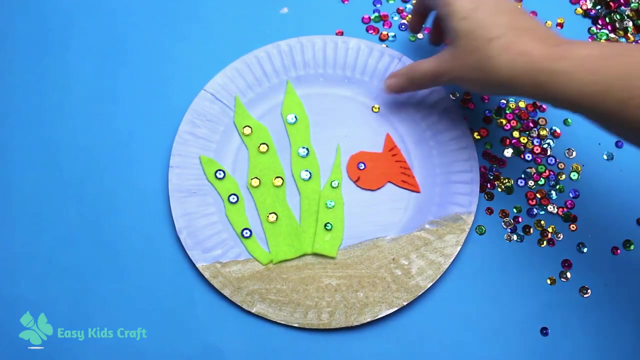 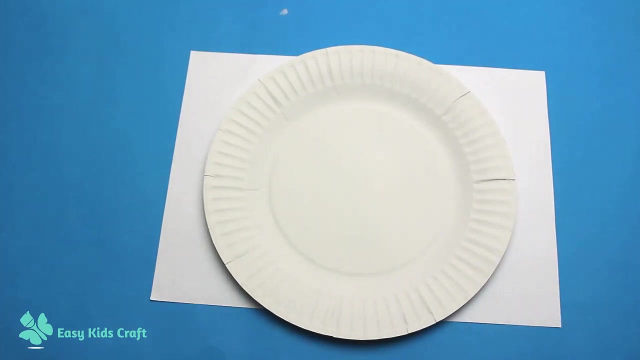 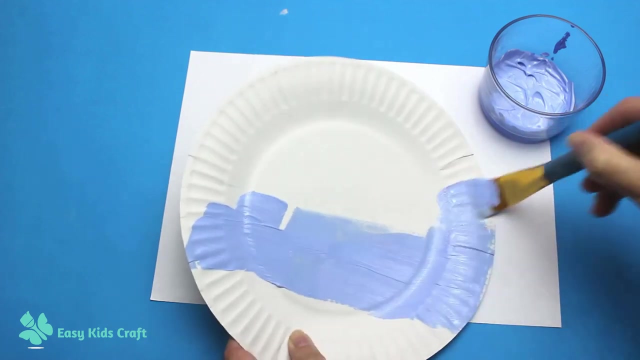 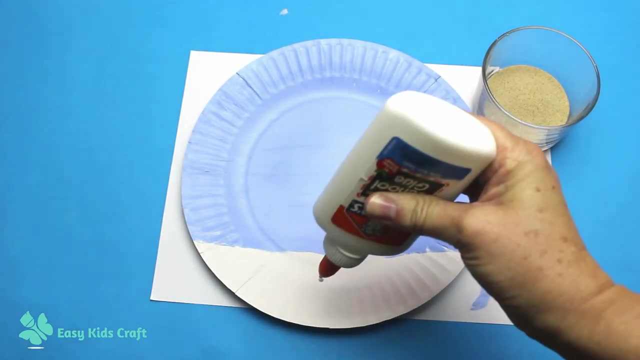 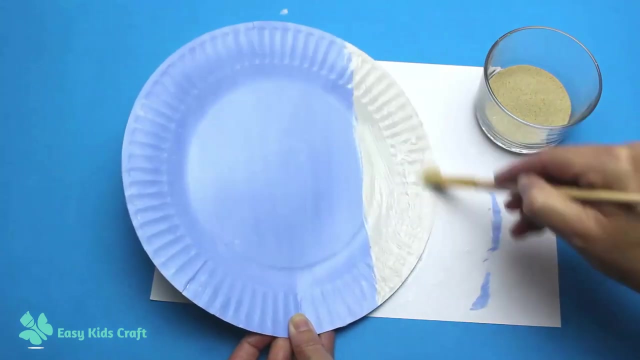 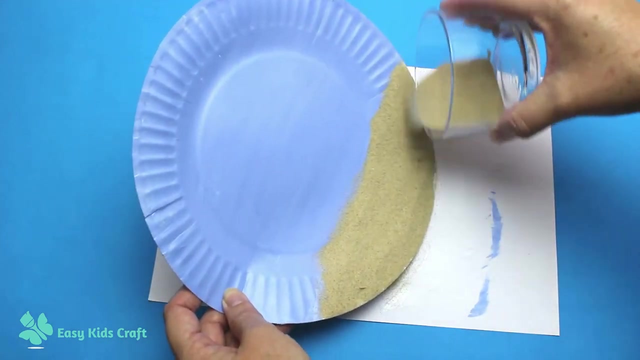 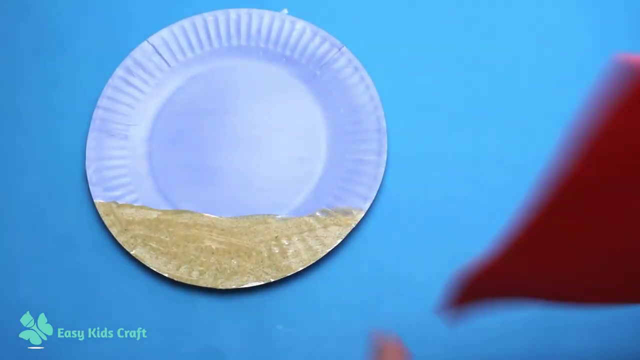 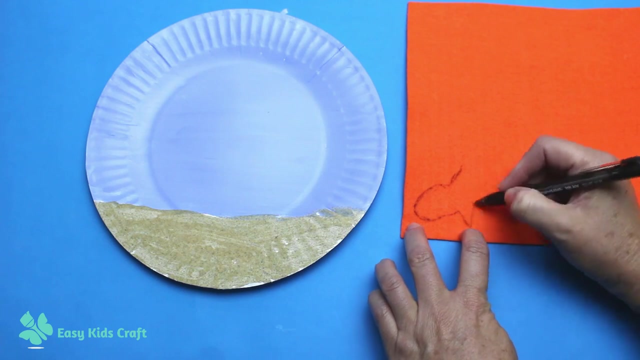 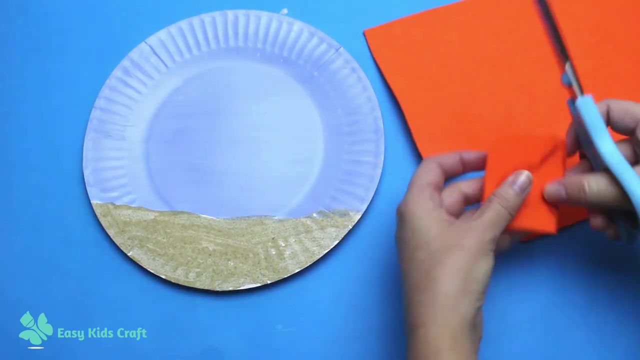 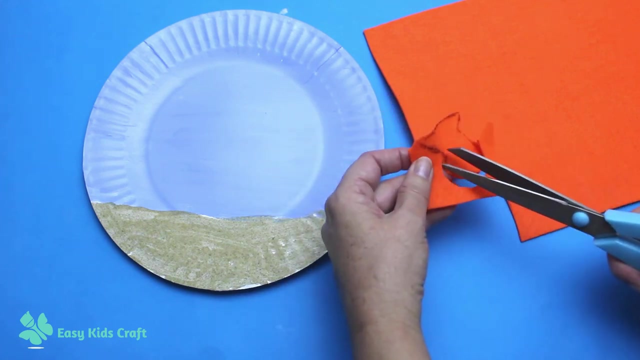 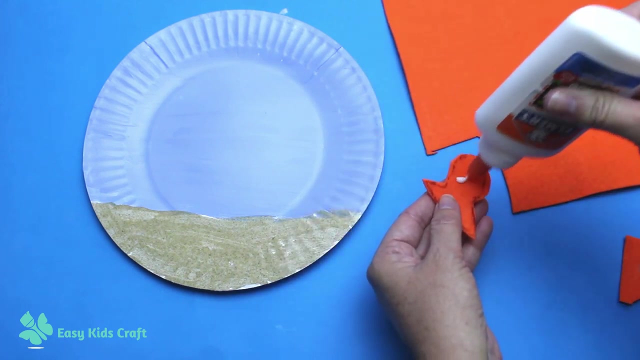 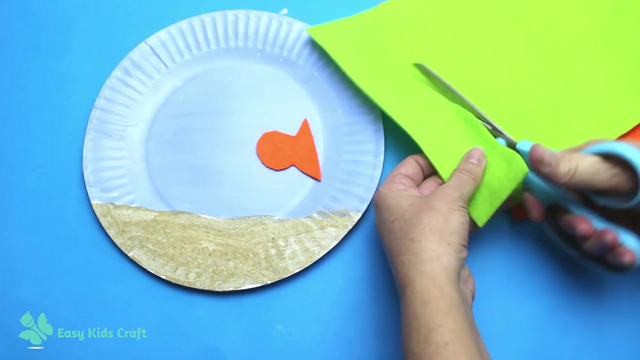 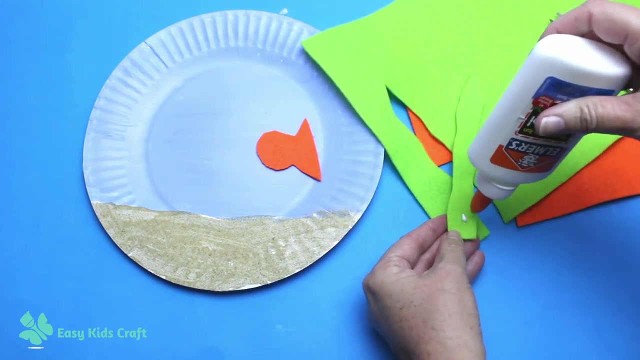 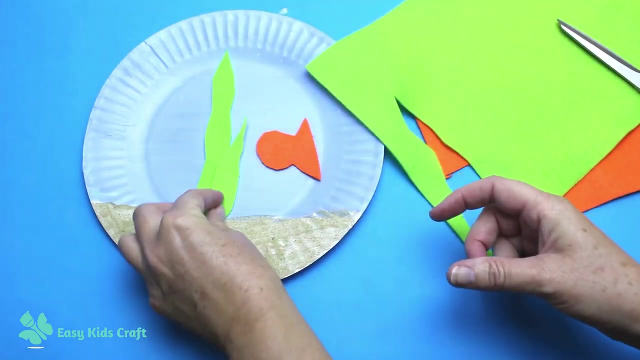 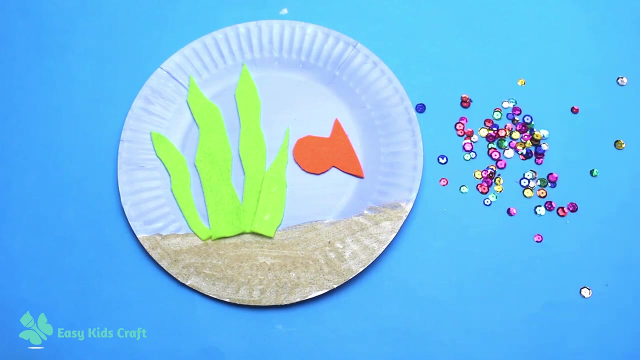 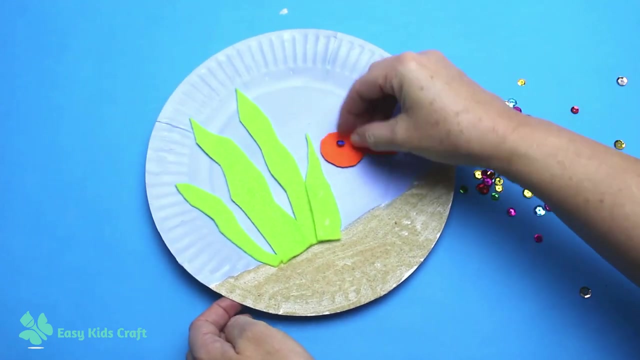 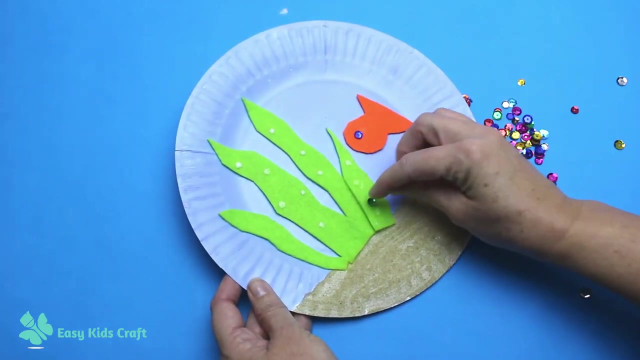 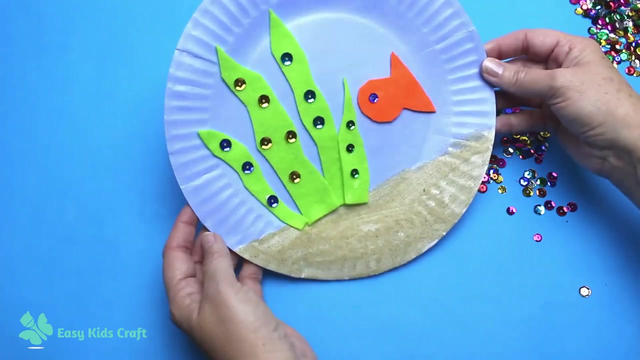 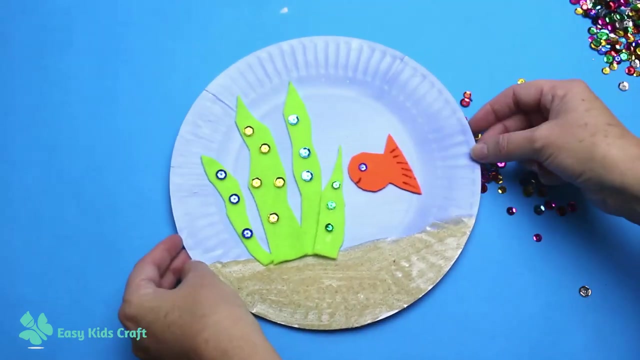 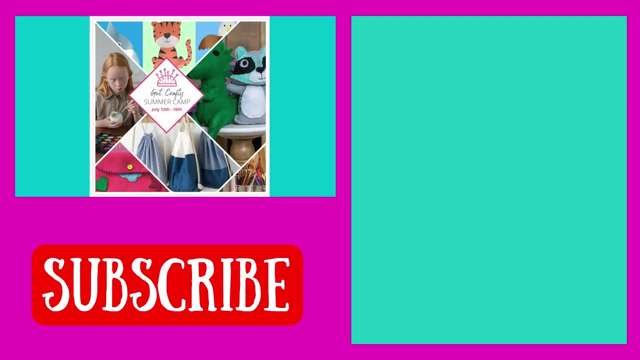 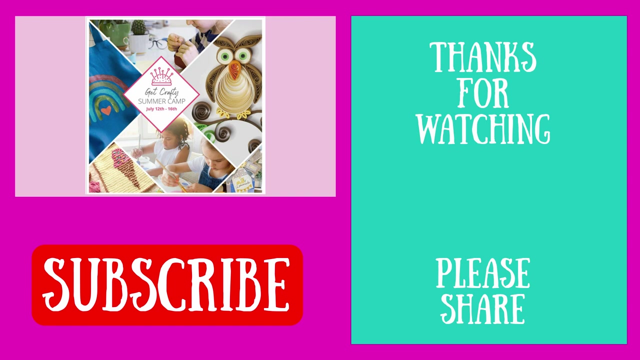